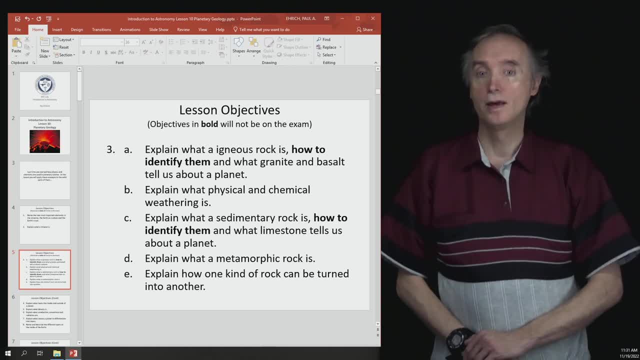 particular, you should know about lime salt. So there you go. You've figured out a little bit about what atmospheric rock is, and then stone. Then explain what a metamorphic rock is, Explain how one kind of a rock can be turned into another kind of a rock, given the right pressures and temperatures and compositions. 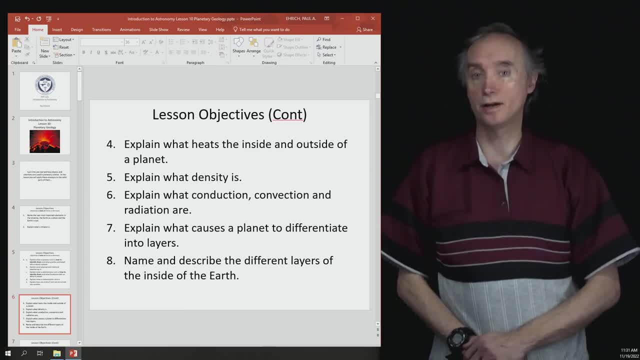 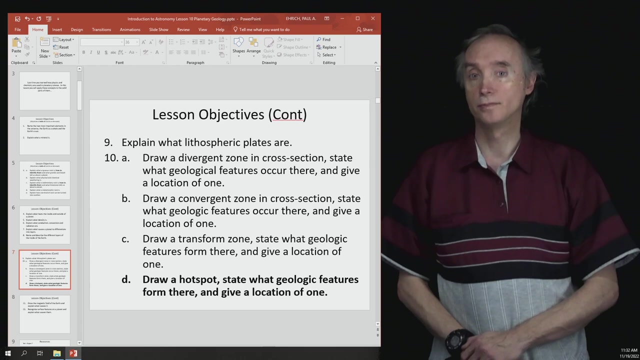 Explain what is it that heats up the inside and the outside of a planet. Explain the concept of density. Explain what heat conduction, convection and radiation are. Explain what causes a planet to differentiate into different layers. Name and describe the different layers of the inside of the earth. Explain what lithospheric plates are, Then be able to draw a divergent. 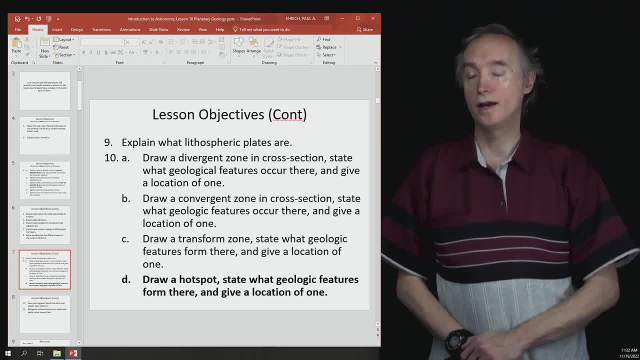 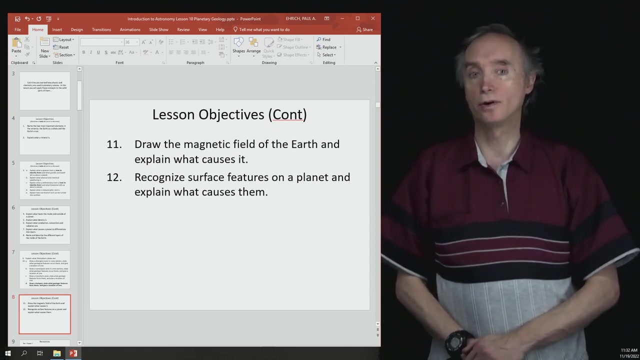 zone, A convergent zone and a transform zone- and be able to explain the different kinds of geological features that are created by each of these different kinds of plate interactions. And then also, you should know what a hotspot is And then be able to draw the magnetic field of the Earth and explain what causes it. and 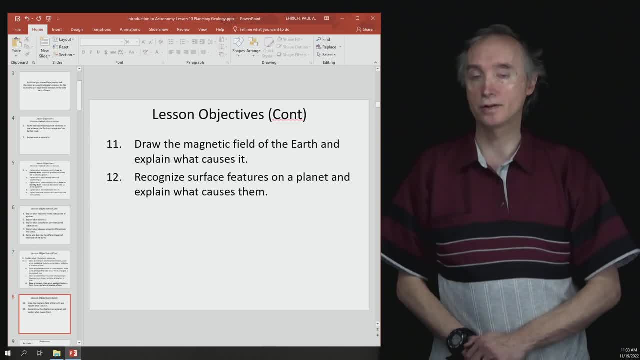 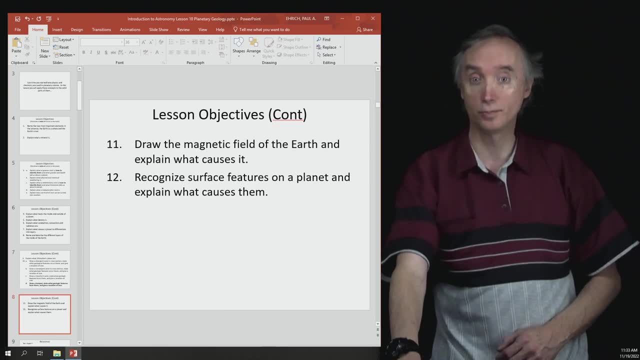 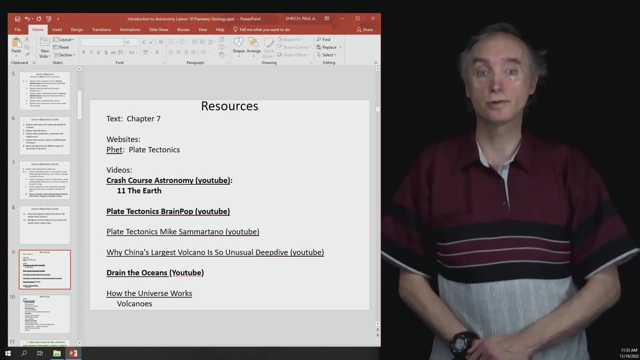 then recognize different surface features on a planet and explain what causes them. So this is a pretty extensive lesson and we're going to break this down into a whole bunch of little pieces. So your resources, So in your textbook, read chapter 7, and then you'll notice that there is a whole lot of 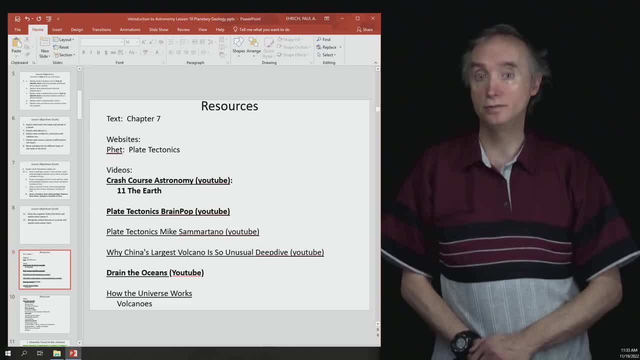 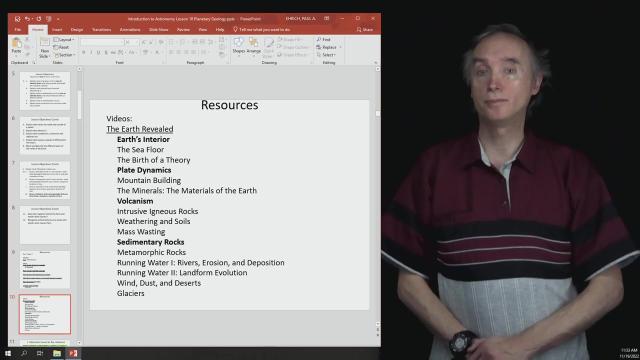 different videos that you can be watching on geology. So there is a crash course, First episode, crash course- astronomy on the Earth, And then there is a video on YouTube called plate tectonics- brain pop. that might be interesting And that, but there is a complete video series on geology. if you're interested in this, 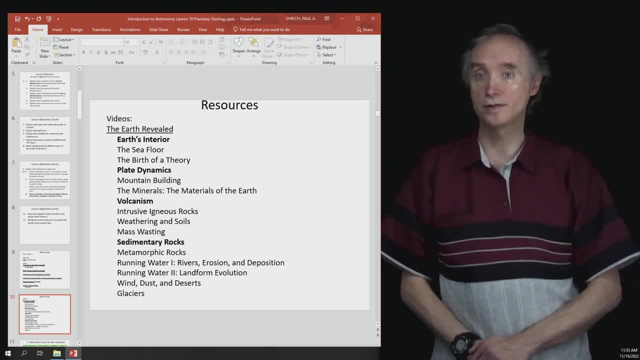 So this is found at the Earth Revealed And this is found W? dot learner dot org and you'll find this complete video series. each of these videos is about 30 minutes long and it covers every aspect of geology. Now we're only going to be interested in one of these. 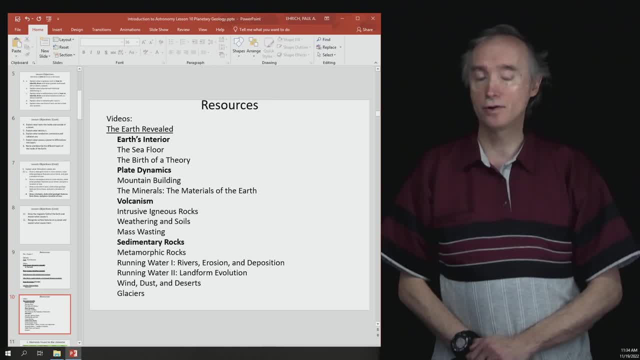 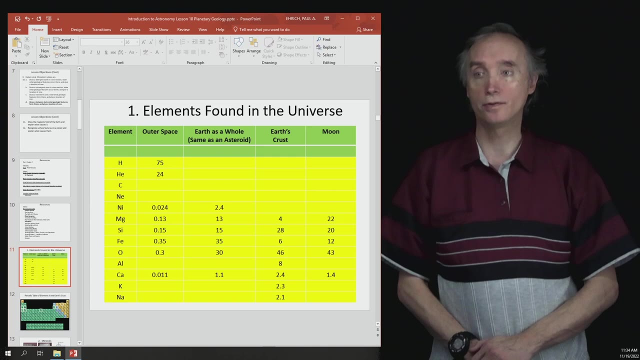 The one that says plate dynamics. So if there's any of those videos that you should be watching, it would be that one. But if you like this geology stuff, feel free to watch the rest of those videos. Okay, we're going to take a break and when we come back we're going to start with. well, 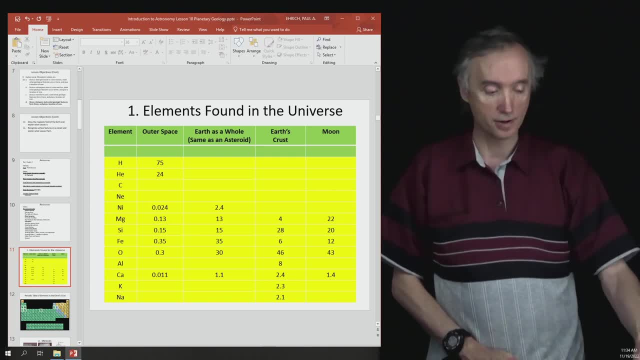 what are starting elements to begin with? I'll see you in just a moment. 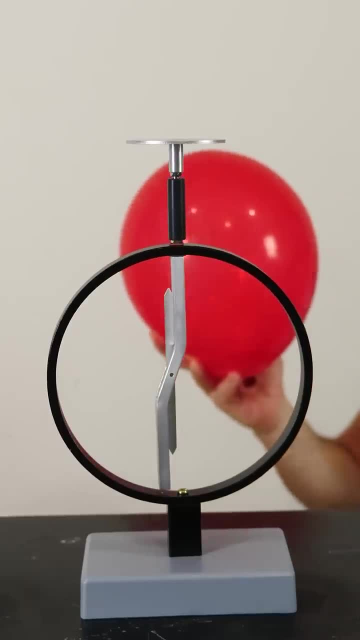 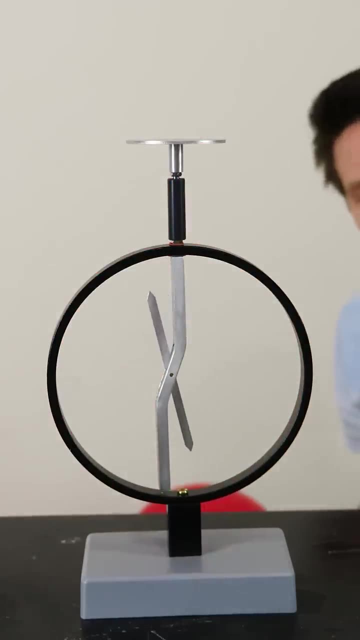 This is an electroscope. You can trap charges on the top plate and this makes the needle move away from the center. So if I take a balloon and rub it on my head- it's actually scraping electrons off my hair- Then I can deposit them on the plate and charge it up If I touch the plate. 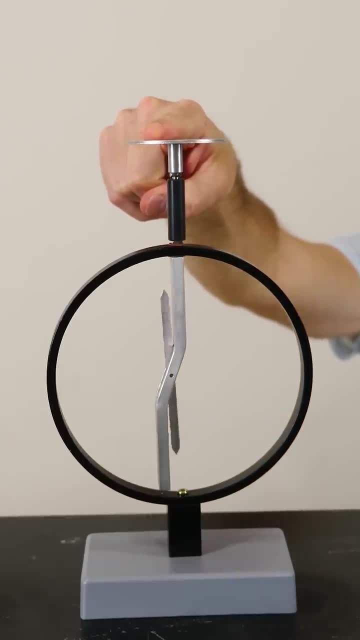 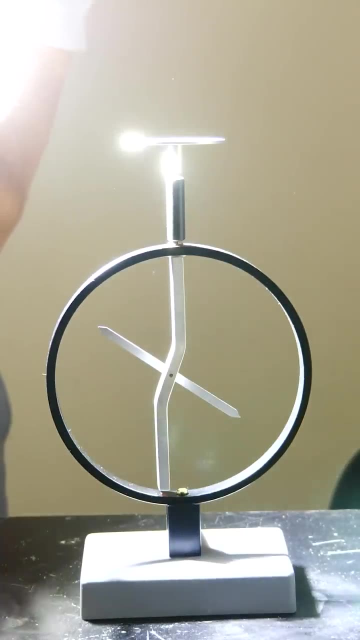 the electrons escape back to my body, But if we don't touch it it stays charged. Now, if I shine trillions of photons on the plate from this 100,000 lumen flashlight, it can't knock any electrons loose. If light only acted like waves, really bright, visible light should have been able. 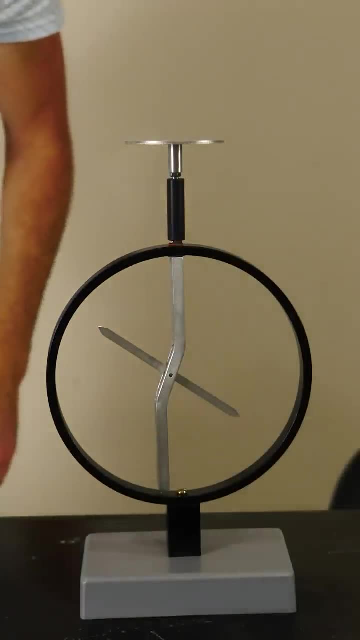 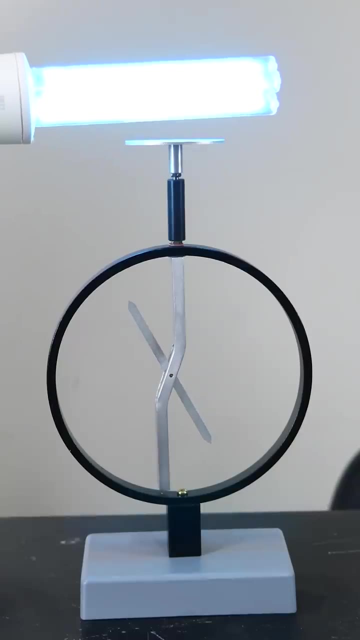 to knock the electrons off. But we know light acts like particles as well, where each individual photon has to have enough energy to knock the electrons off. But if I take a dimmer UV-C light, the photons have enough energy to knock electrons off the plate and discharge it. But if I charge it, 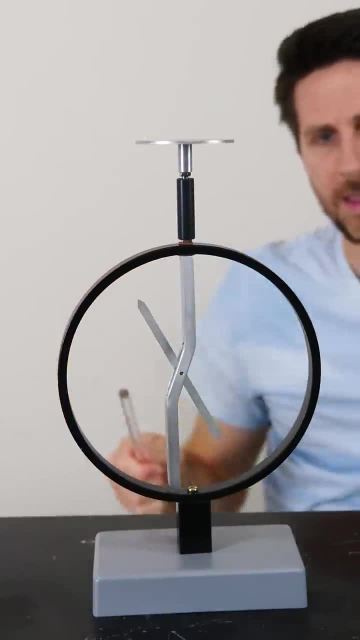 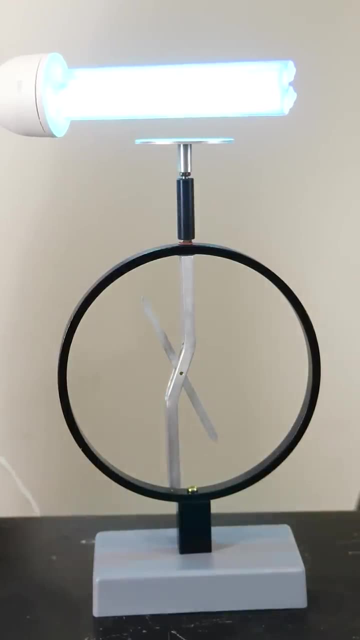 with a positive charge instead. so now I'm removing electrons this time. then the UV-C light doesn't do anything, because it can't knock protons off the plate. Those are too big. What you just saw is called the photoelectric effect. It won Albert Einstein the Nobel Prize and proved that light.